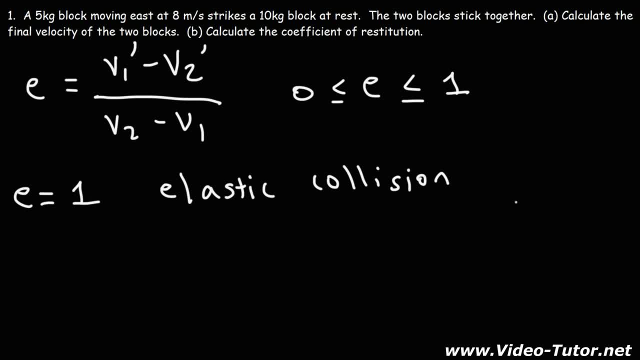 But for an elastic collision the kinetic energy is conserved. So there's no loss of kinetic energy for these types of collisions, When the coefficient of restitution is equal to 0, you have what is known as a completely inelastic collision. For all types of collisions, momentum is conserved. 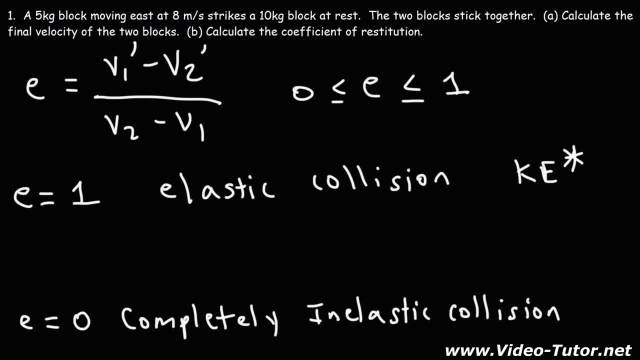 For an inelastic collision, kinetic energy is not conserved. Now, if the coefficient of restitution is equal to 0, you're dealing with a completely inelastic collision. When the coefficient of restitution is between 0 and 1, you just have a regular inelastic collision. 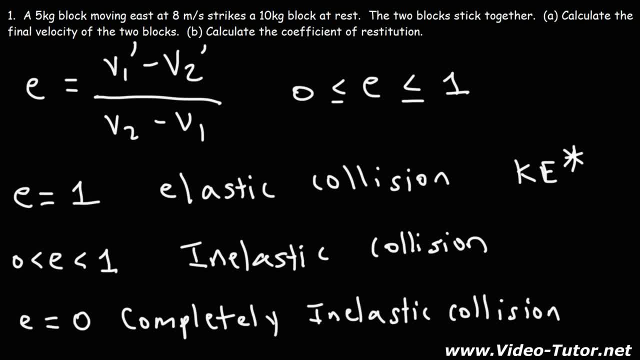 So that's what the coefficient of restitution will tell you. It will tell you if the collision is elastic or if it's inelastic, and to what degree is it inelastic? Is it completely inelastic or partially inelastic? So now let's work on some practice problems. 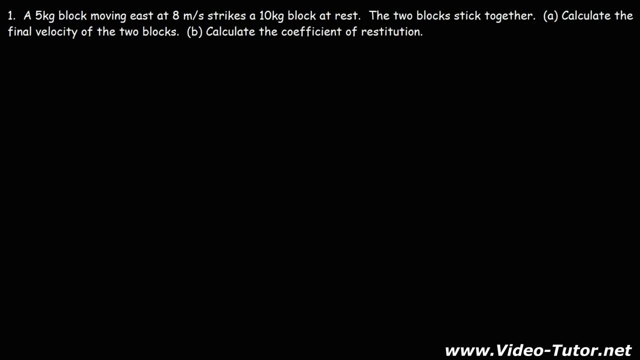 Let's start with this one. A 5 kg block moving east at 8 m per second strikes a 10 kg block at rest. So let's draw a picture, So let's say: this is the 5 kg block and it's moving east. 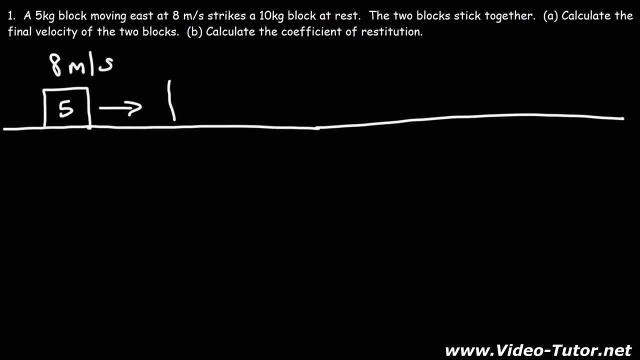 At 8 m per second and it's going to strike a 10 kg block and that block is at rest. Now, after the collision, these two blocks, they will be sticking together And in part A we'll need to find a combined final velocity of the two blocks. 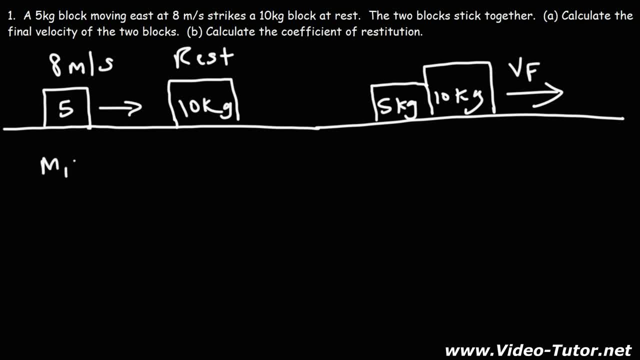 Let's do this. So the initial momentum, that is, the total momentum before the collision, is going to be m1 v1 plus m2 v2.. And that's going to equal the final momentum, which is going to be the sum of the two masses multiplied by their common final velocity. 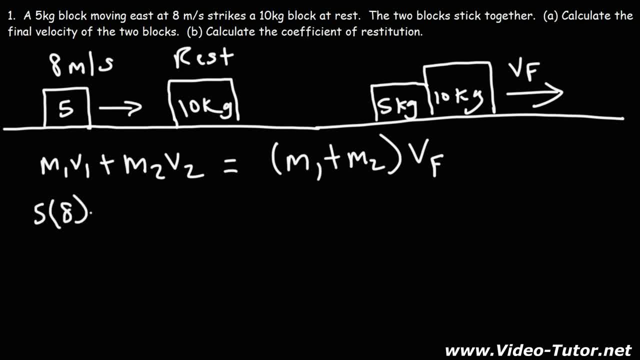 Now m1 is 5 kg, v1 is 8, m2 is 10, v2 is 0.. Now m1 plus m2, 5 plus 10 is 15. And we can solve for v final. So 5 times 8 is 40.. 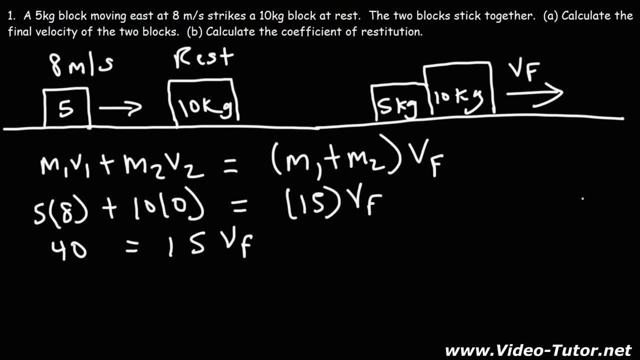 And that's equal to 15 vf. So v final is going to be 40 divided by 15.. That's 8 over 3, which you can round that to 2.67 m per second. So that's the answer for part A. 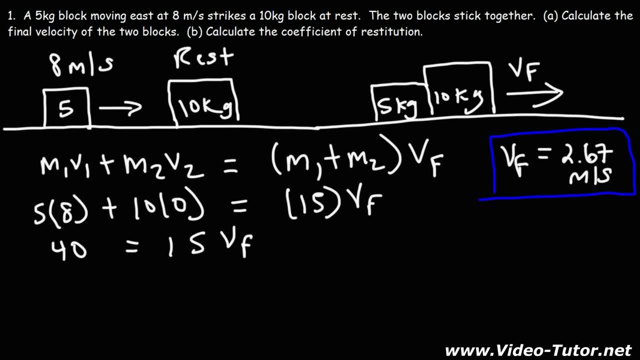 Now part B: Calculate the coefficient of resistance. So that's going to be v1 prime minus v2 prime over v2 minus v1.. So v1 prime and v2 prime the final velocities of the two blocks. because they're sticking together, they're moving at the same speed. 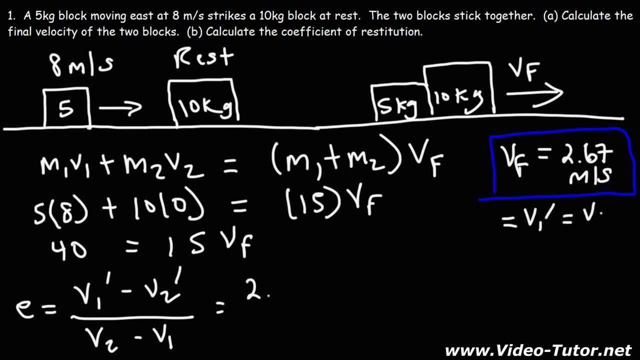 So v1 prime and v2 prime. they're both equal to 2.67.. Now v2 was at rest, so that was 0.. V1 was 8.. So because the two blocks are sticking together and they're moving at the same speed, the coefficient of restitution will be 0.. 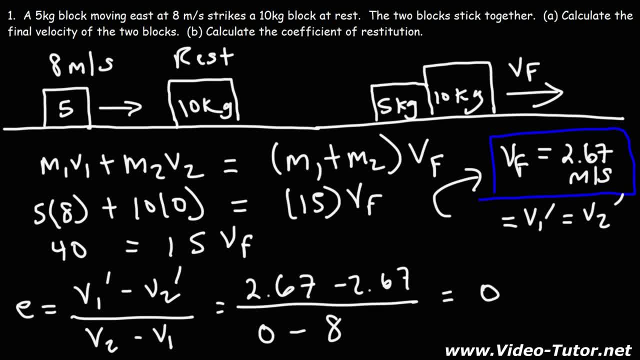 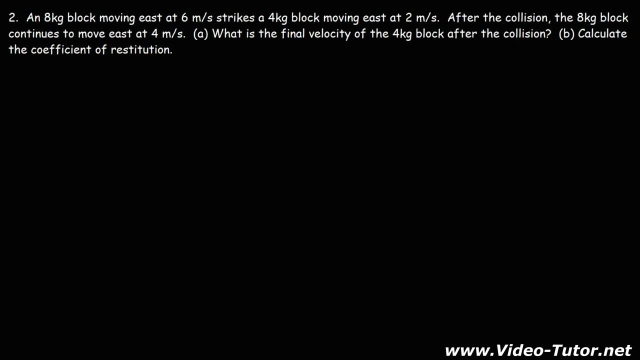 Because these two they will cancel out. So what this tells us is that we're dealing with a completely inelastic collision, So you're always going to have that situation whenever the two blocks stick together. Number two: an 8 kg block moving east at 6 m per second strikes a 4 kg block moving east at 2 m per second. 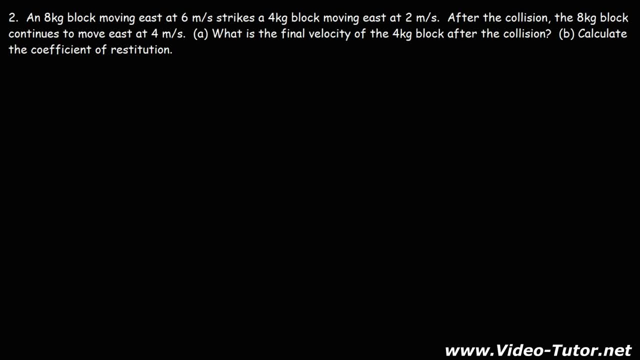 After the collision, the 8 kg block continues to move east at 4 m per second. What is the final velocity of the 4 kg block after the collision? So here is the final velocity of the 4 kg block after the collision. 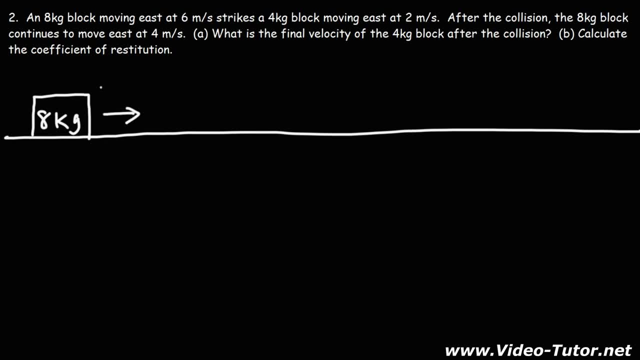 So here is the 8 kg block and it's moving east at 6 m per second. And here we have another block. it's a 4 kg block, but this one is moving east at 2 m per second. Now, after the collision, the 8 kg block is moving east, but at a lower speed, at 4 m per second. 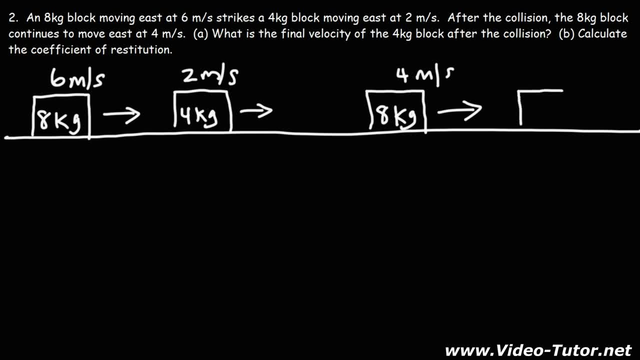 So it lost some energy. We need to find the final velocity of the 4 kg block And then we can move on to part B. So this is v1,, this is v2,, this is v1'. We need to find v2'. 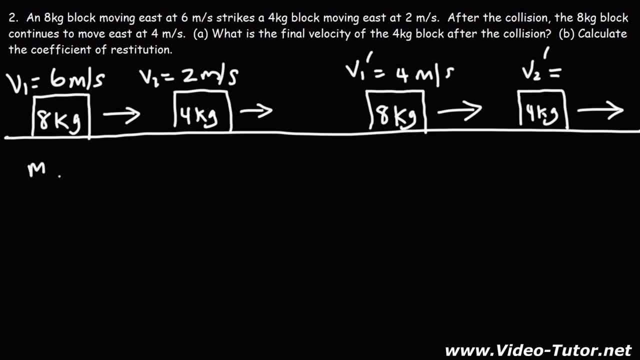 So we have m1v1 plus m2v2.. So that's going to equal m1v1'. So m1 is 8, v1 is 6, m2 is 4, v2 is 2.. m1 is 8, v1' is 4, m2 is 4, and let's solve for v2'. 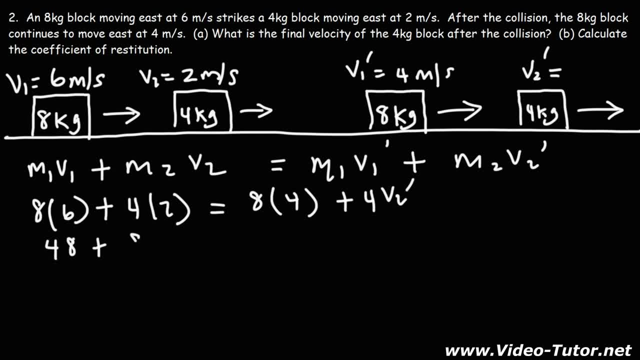 So 8 times 6 is 48,, 4 times 2 is 8,, 8 times 4 is 32.. And then 8 plus 48.. 8 plus 48. That's going to be 56.. 56 minus 32 is 24.. 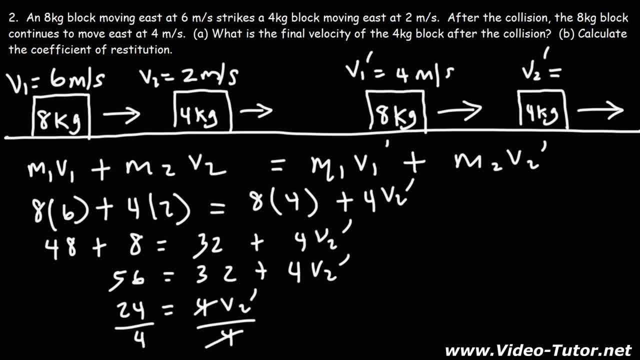 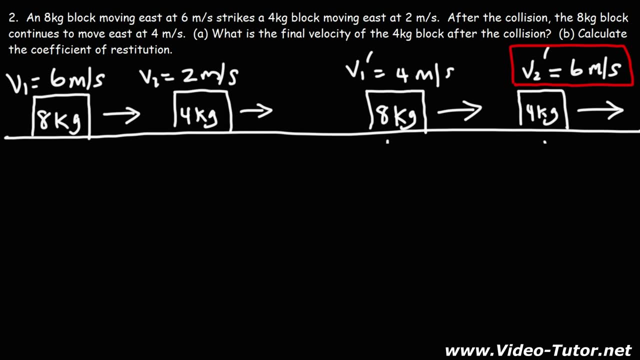 And dividing both sides by 4, we have 24 over 4, which gives us 6 m per second. So that's the final velocity of the 4 kg block after the collision. Notice that these two blocks, they are not sticking together. 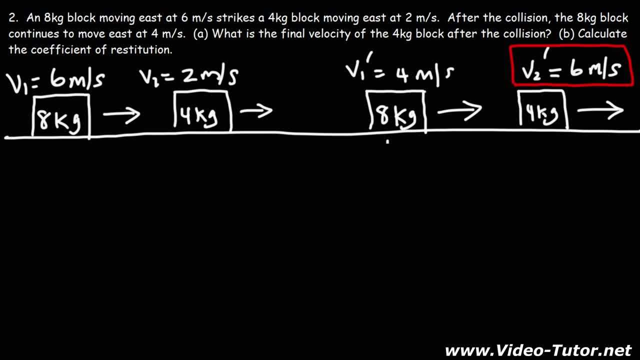 So because they have, because after the collision, because they have different speeds and they're not sticking together, this will not be a completely inelastic collision, but it will simply be just an inelastic collision. So let's calculate the coefficient of restitution. 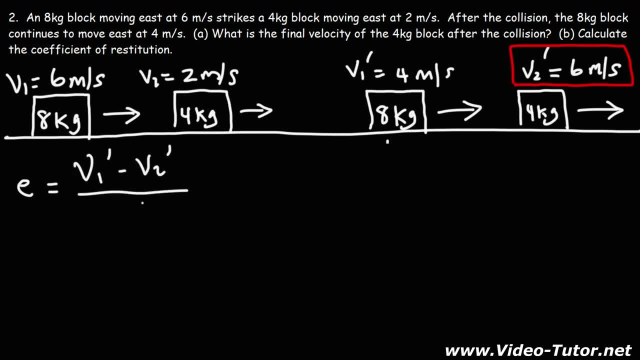 So it's going to be v1' minus v2' over v2 minus v1. So v1' is 4, v2' is 6, v2 is 2, and v1 is 6.. So 4 minus 6 is negative 2, 2 minus 6 is negative 4.. 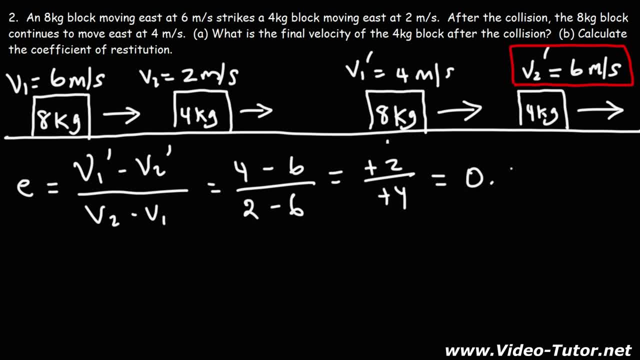 The negatives cancel. 2 over 4 is 0.5.. So this is a value between 0 and 1.. So that tells us that the collision is simply an inelastic collision. It's not an elastic collision, nor is it a completely inelastic collision. 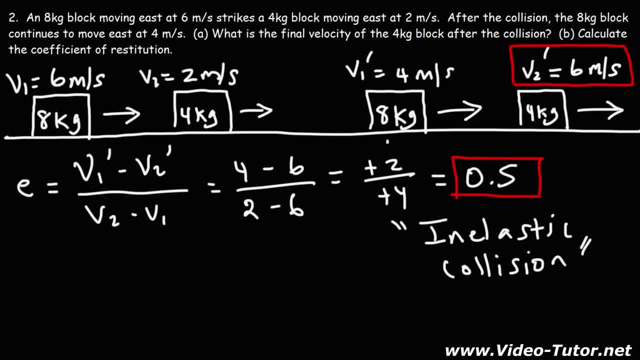 It's simply an inelastic collision. Now we can see if we have an inelastic collision by checking if the kinetic energy has been conserved or not. For an inelastic collision, the kinetic energy is not conserved, So the kinetic energy is going to be 1 half mv squared. 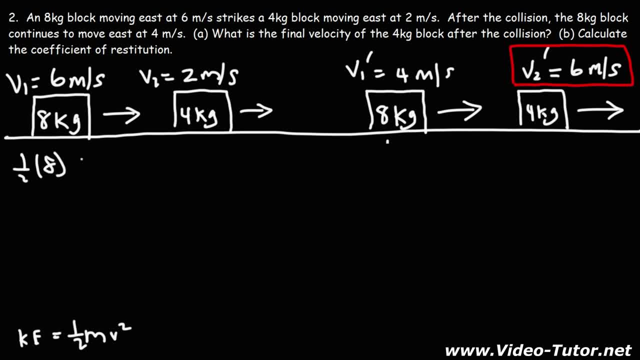 So for the first one, it's going to be: 1 half 8 times 6 squared, Half of 8 is 4, so 4 times 6 squared that's 144 joules. Now for the second one, it's going to be: 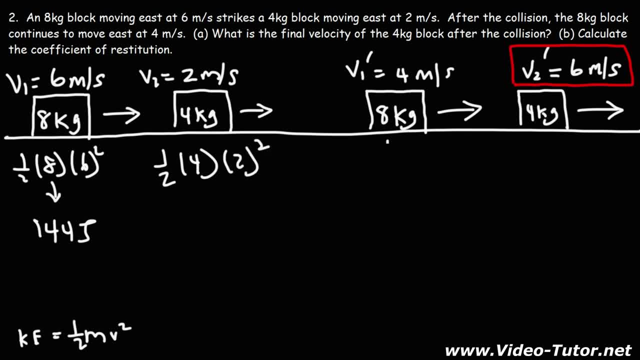 1 half times 4 times 2 squared. Half of 4 is 2, 2 times 2 squared, that's 2 times 4, which is 8.. For the next one, it's 1 half times 8 times 4 squared. 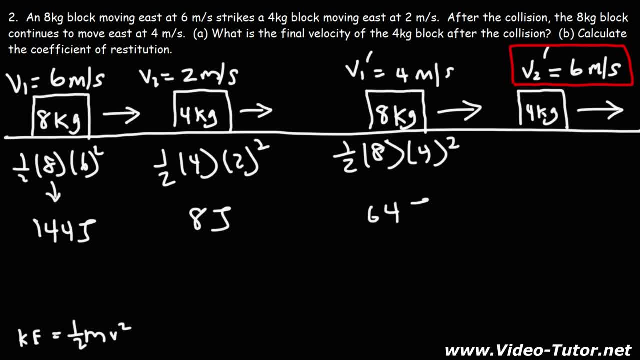 So that's going to be to be 64 joules. and for the last one, half of 4 is 2, 6 squared is 36, 2 times 36 is 72. So if we calculate the total before the collision, it's 144 plus 8, which is 152 joules, and 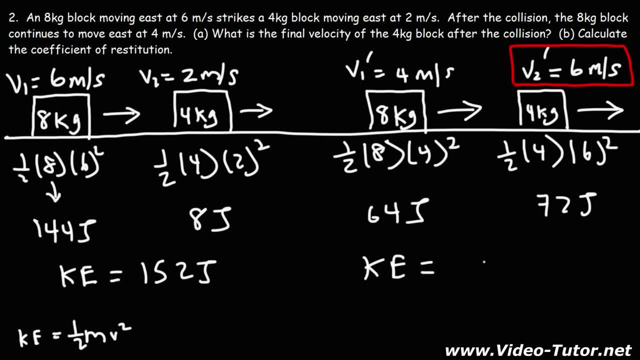 after the collision it's 64 plus 72, which is 136 joules. So we could see that we have a loss of negative 16 joules of kinetic energy. So because there was a loss of kinetic energy, we know that we're dealing with an inelastic. 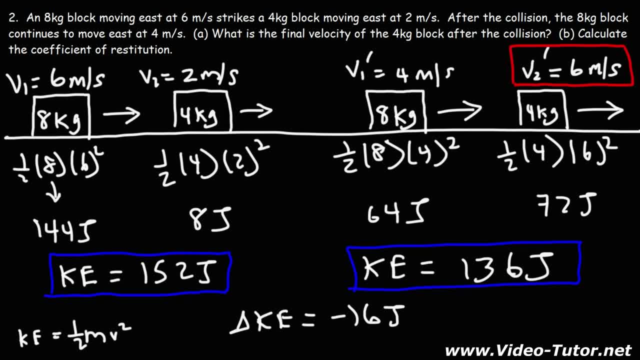 collision. Now, if you were to follow the same procedure for the last problem, the loss in kinetic energy is about 53.5 joules when the coefficient of restitution is 0. For this problem there was only negative 16 joules of energy loss and the coefficient 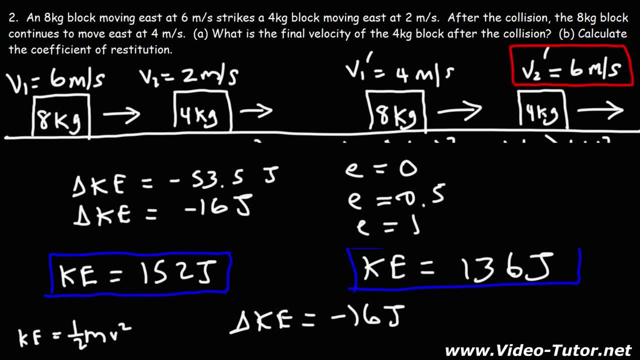 of restitution is 0.5. And when it's 1, we know that we're going to have a perfectly elastic collision. There will be no loss of kinetic energy. So, generally speaking, as the coefficient of restitution increases from 0 to 1, the loss of kinetic energy goes. 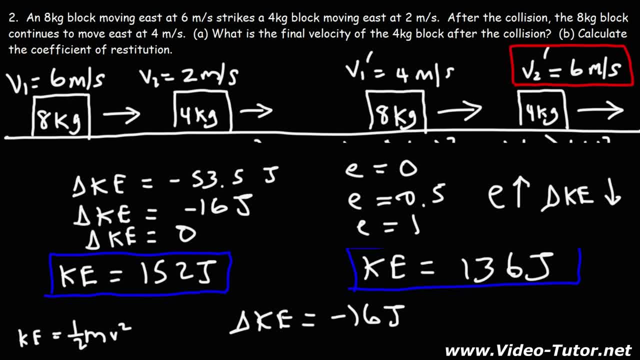 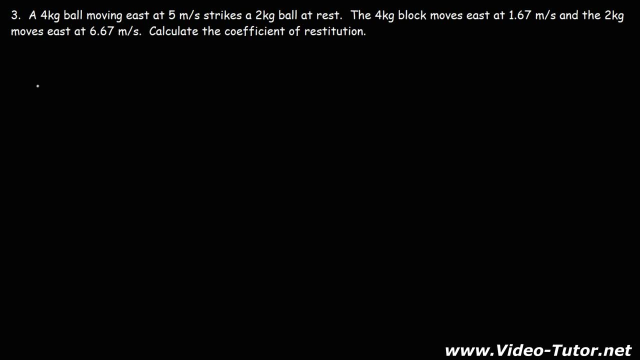 down. As E goes up to 1, the loss of kinetic energy goes down to 0.. Now let's work on this problem. So we have a 4-kilogram ball and it's moving east at 5 meters per second and it strikes. 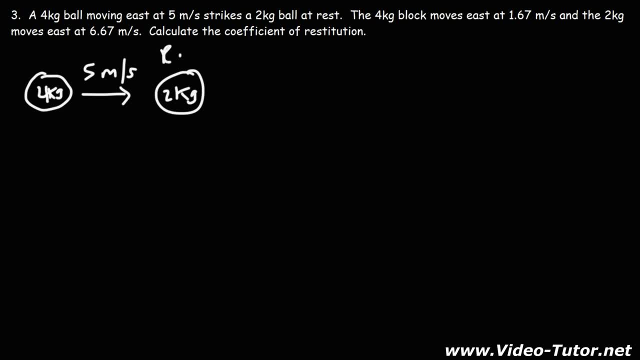 a 2-kilogram ball which is at rest Now, the 4-kilogram ball after the collision. it's going to move east at 1.67 meters per second, And a 2-kilogram ball is going to move east at a higher speed, at 6.67 meters per second. 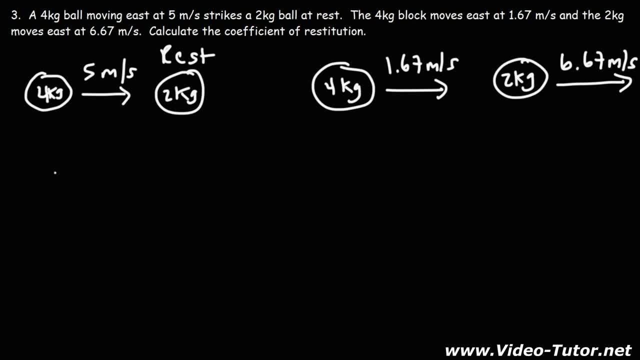 Calculate the coefficient of restitution. So it's going to be V1 prime minus V2 prime over V2 minus V1.. So this is V1, V2 is 0, this is V1 prime and this is V2 prime. 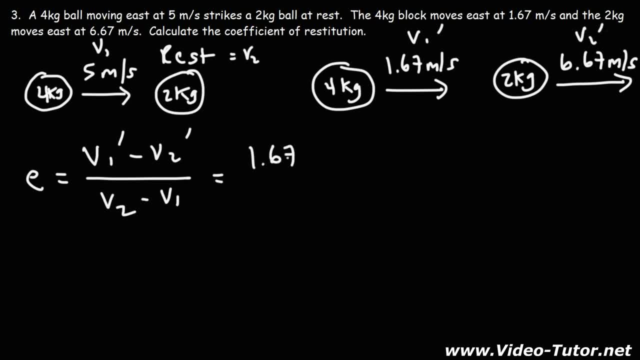 So V1 prime in this problem is 1.67, V2 prime is 6.67,. V2, the 2-kilogram ball is at rest, so that's 0, and V1, that's going to be 5.. 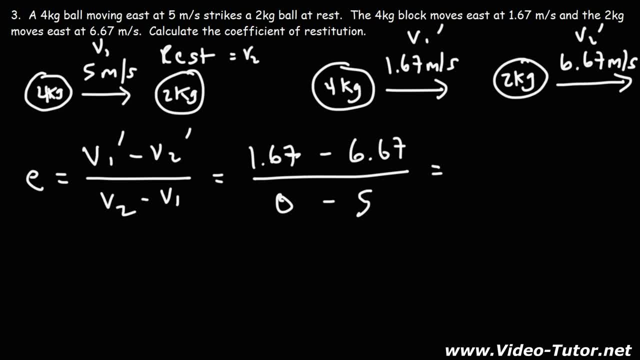 So 1.67 minus 6.67, that's negative 5, 0 minus 5 is negative 5, which is 1.. So, because the coefficient of restitution is 1, what we have here is a perfectly elastic collision. 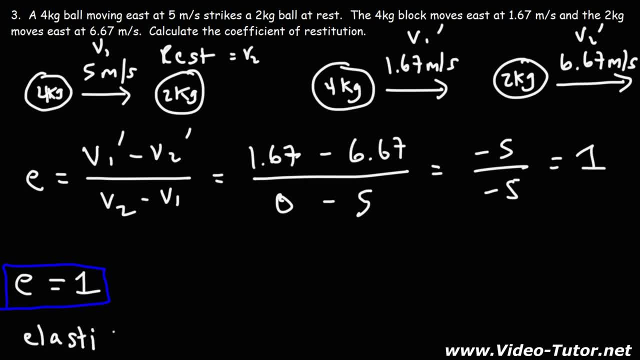 So because we have an elastic collision, we know that the kinetic energy is going to be conserved, So there's no loss in kinetic energy And we can go ahead and determine that in this problem. So if we calculate the kinetic energy for the first ball, 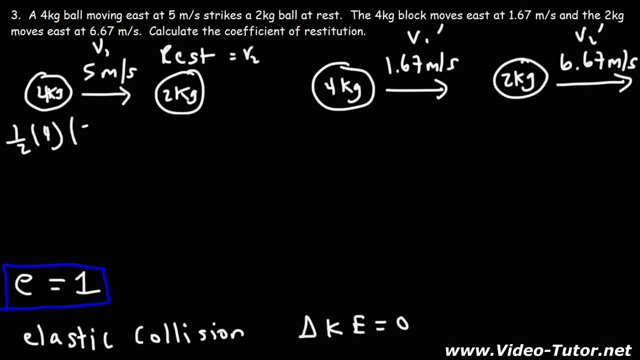 it's going to be 1 half times 4 times 5 squared. Half of 4 is 2, 5 squared is 25, 2 times 25 is 50.. Now for the second ball. it's not moving, it's at rest, so it has no kinetic energy.